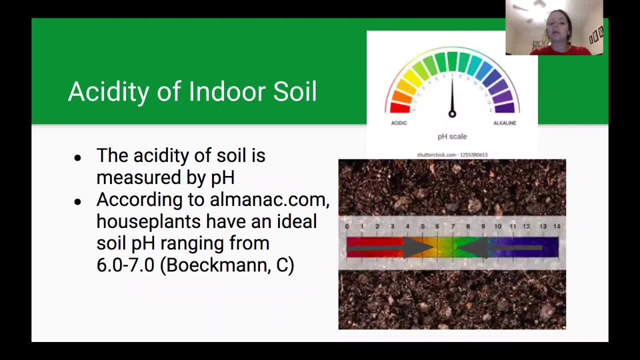 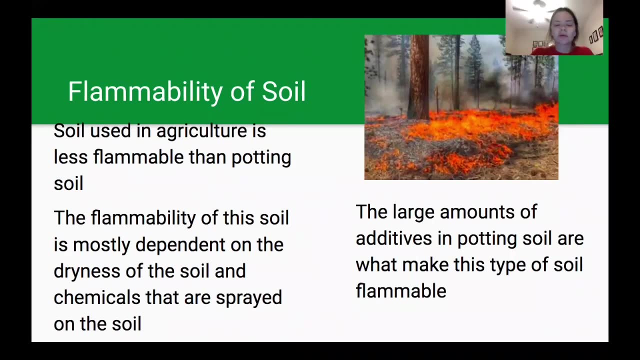 measured through pH, and according to almanaccom, houseplants and indoor soil have an ideal soil pH ranging from 6.0 to 7.0.. Next up is the flammability of soil, So in this one, we compared agricultural soil to indoor potting soil. 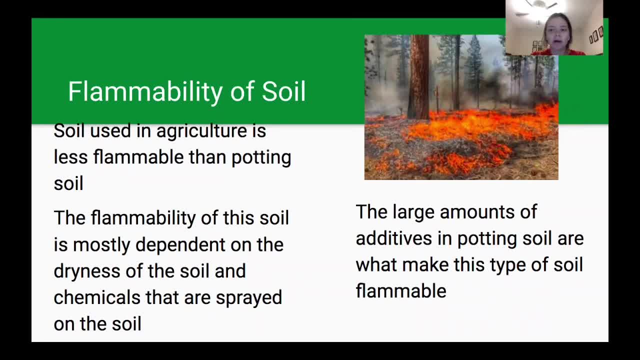 So agricultural soil is less flammable than potting soil, and the flammability of agricultural soil is mostly dependent on the dryness of the soil and some of the chemicals that are sprayed on it or mixed in with it, And then some of the reasons that potting soil is so flammable. 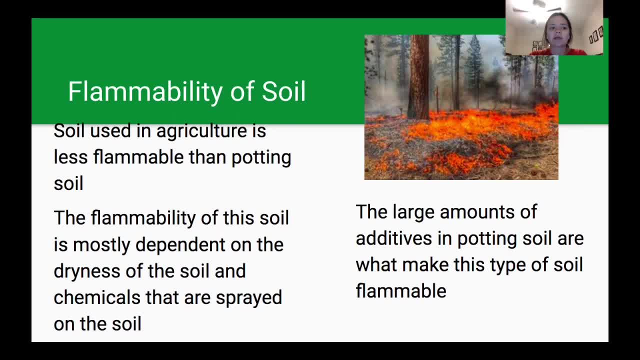 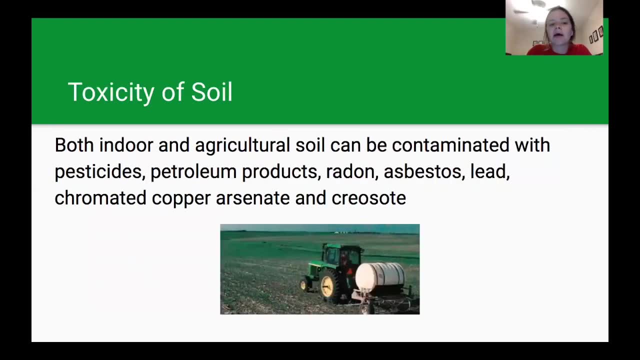 more so than agricultural soil is because of the additives. Some of the ingredients that are mixed in include peat, moss, shredded wood, bark, styrofoam and vermiculite, And then after that, we looked at the toxicity of soil. 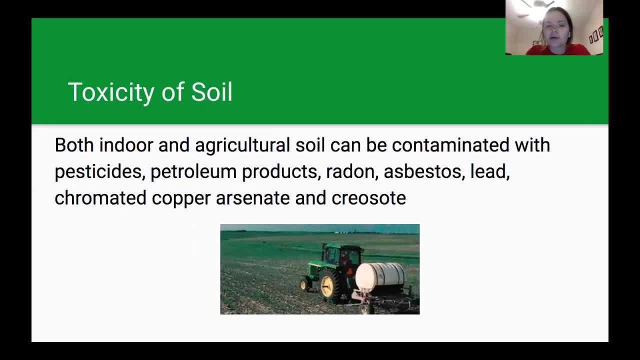 So these indoor and agricultural soils are pretty similar in this: They can both be contaminated with pesticides, petroleum products, radon, asbestos, lead, chromated copper, arsenate and cressoate And less split in parts, And this toxicity not only affects the soil, but it can transfer to foods that is grown. 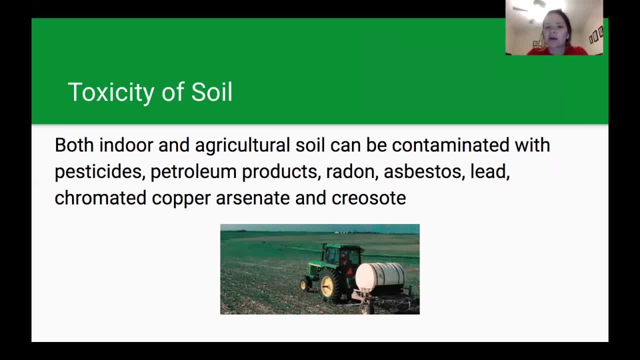 within it or plants that are grown within it, And then, in turn, can affect, you know, either animals that eat that food or even people who eat the food or you know could interact with some plants, smile, some flowers, something, 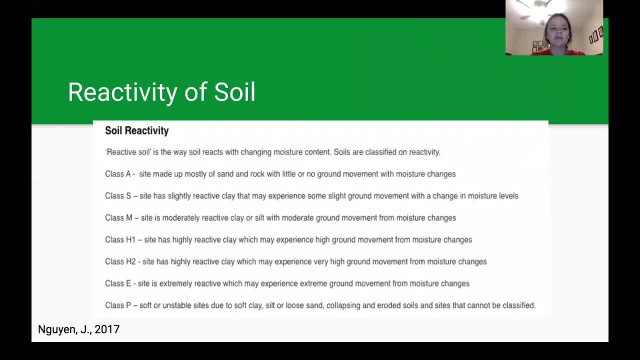 like that. And then the last chemical property that we looked at was the reactivity of soil. So one type of soil reactivity looks at how soil reacts in changes. Next up to событи will be the assignment of soil, meaning the pump, True beginners. 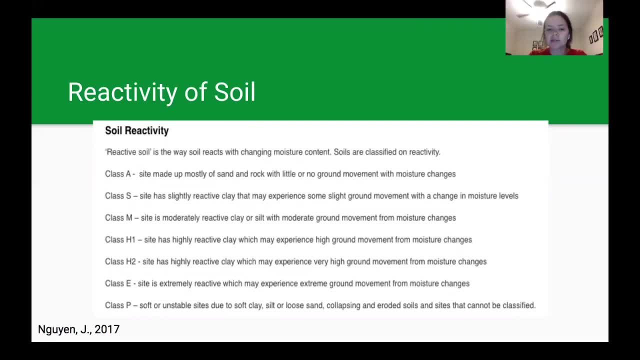 So we'll take a look at this as well, And I'm looking for groups that just want to pop a slide. Y'all want to put your questions will. changes to different moisture contents of the soil. So this graphic just shows how they classify. 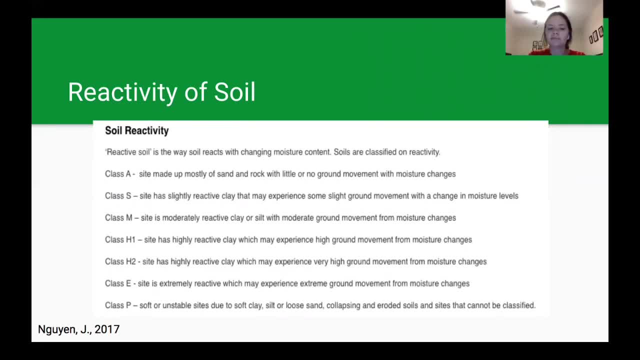 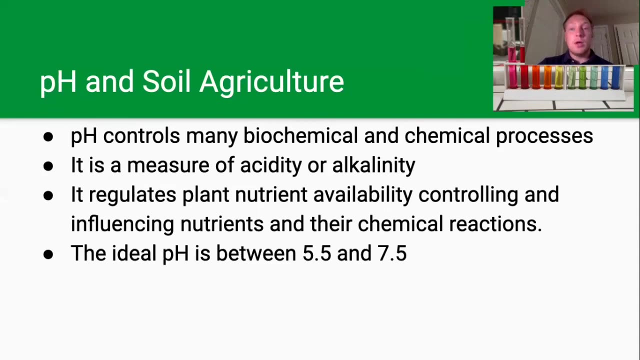 it So class, and then a letter, sometimes a number just kind of goes over how they classify each soil and then you know based on the moisture content and how it changes as the moisture changes. And next up we have Jordan pH and soil agriculture. pH is very important because it controls many 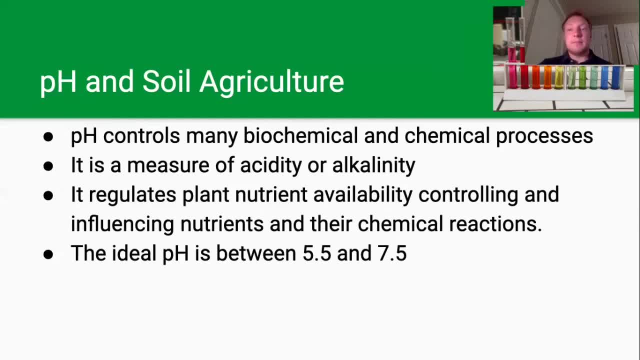 biochemical and chemical processes operating within the soil. It is a measure of acidity or alkalinity. It regulates plant nutrient availability by controlling and influencing nutrients and their chemical reactions. This means soil and crop productivities are linked to pH. The ideal pH for most agriculture is between 5.5 and 7.5.. Ion exchange and soil agriculture. Ion exchange is 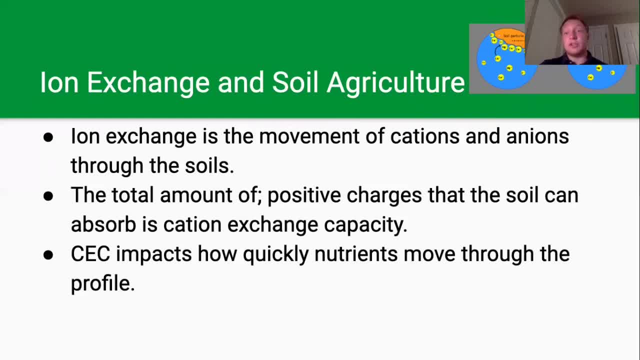 the movement of cations, positive charged elements and anions- negative charged elements- through the soils. The total amount of positive charged elements is the total amount of positive charged elements. The total amount of positive charges that the soil can absorb is cation ion exchange capacity, or CEC. CEC impacts how quickly. 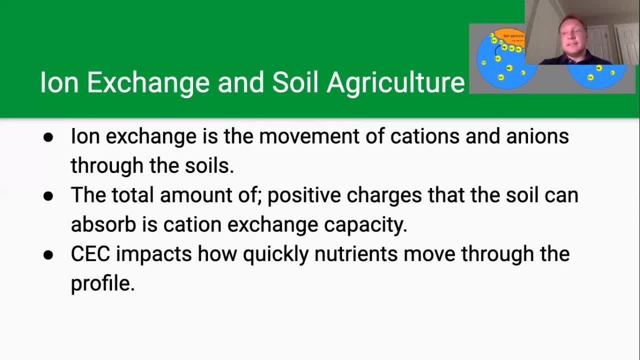 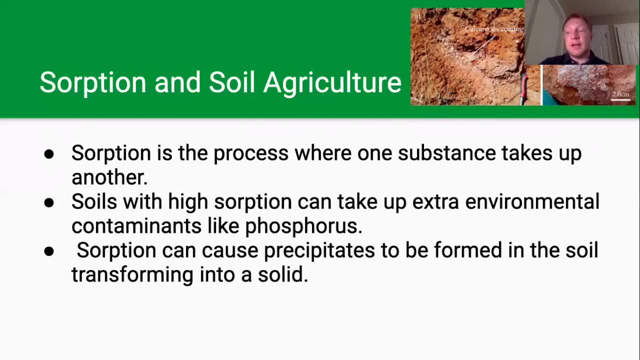 nutrients move through the profile. Soils with low CEC are much less fertile because they can't hold as many nutrients. Sorption and soil agriculture: Soils can capture different nutrients with ions. Sorption is the process where one substance takes up another. Soils with high sorption can take up. 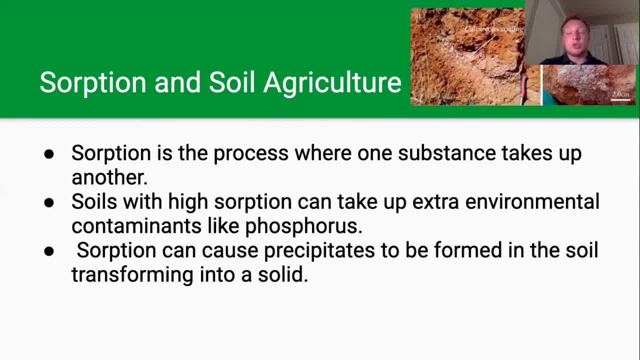 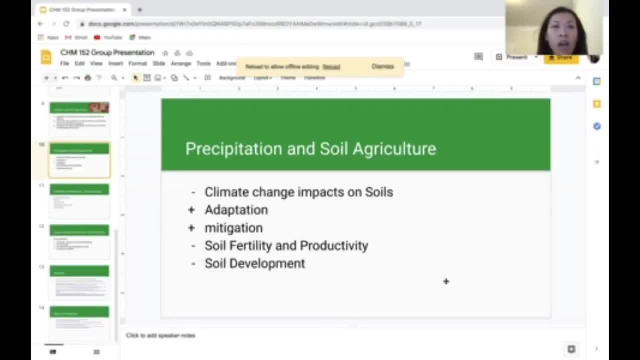 extra environmental contaminants like phosphorus Sorption can cause precipitates to be formed by nutrients or chemicals in the soil, transforming them into a solid. Okay, let's talk about the precipitation of the soil agriculture. So agriculture production depends on weather. Rainfall can either encourage 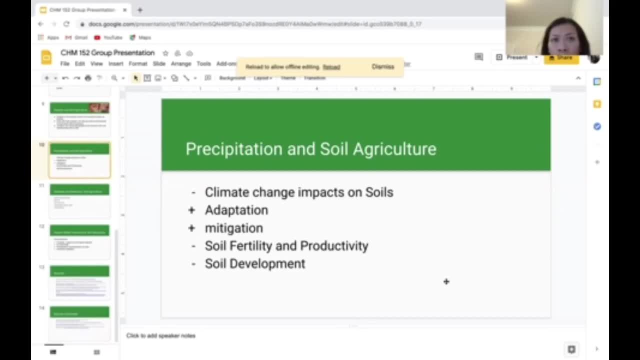 rlaugh or develop crops. Cool temperatures and springtime rains can hinder planting and and seed row just at. hot temperature and drought can adversely stun row or kill mature plants later in the rowing season. Soil is also readily affected by rainfall If it is too wet or too dry. 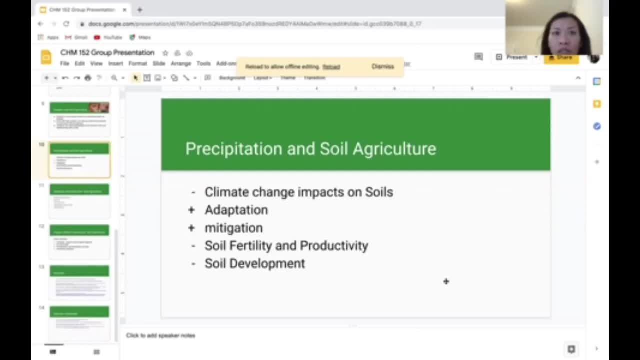 nutrients in the soil can run off and not make it to the plant root, leading to poor row and overall health. Additionally, as mentioned, over watering or too much rain can also lead to bacteria, fungus and moths rowing in the soil. 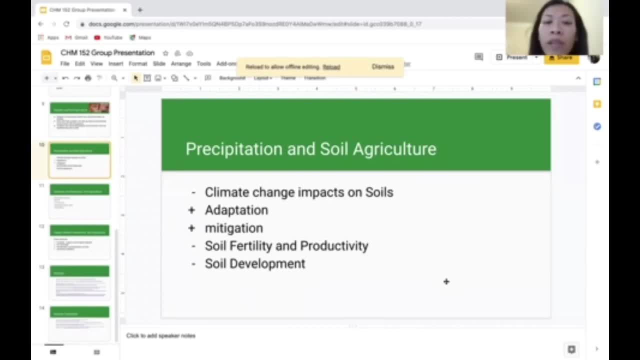 So when the climate change really impacts on soil- especially adaption mitigation and soil for literacy and productivity- and it's in fact to the soil development as well- let's talk about the oxidation and reduction in soil culture. Healthy soils rely on water, oxygen, air and a balanced supply of nutrition. 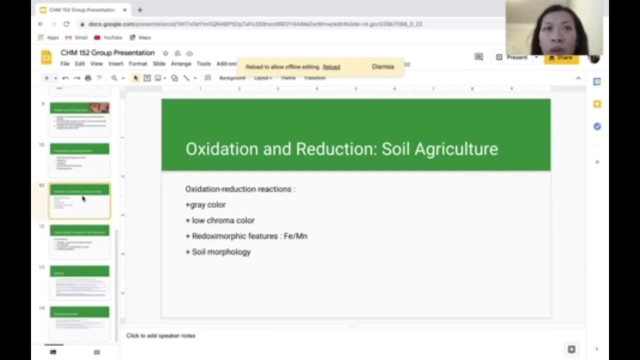 Chemical reaction within the soil can alter the physical structure of available nutrition. Oxidation and reduction process involve the oxygen exchange that takes place between water and in organic materials. These changes affect available nutrition supply. so oxidation Todd appears as a. warum in viro que another? 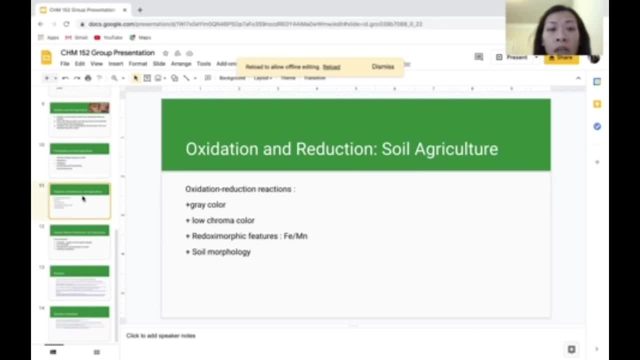 beauty nutritionist began assign a mold. Visambuhan Ash Joel spoke most about in this situation, or not at all. but Aqua, there are plenty of Väk-V Basque terms. it'sipes Noth-I- keluar, it's for basic 뉴�avs. but with my understanding, the various and 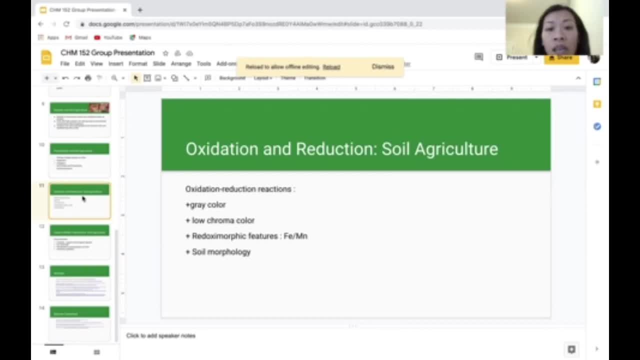 the Experimental advancements and evidence set across the itinerary of the European würden in organic materials. these trends affect available nutrition supply, So the reaction of oxidation and reduction that can happen in the soil can make the soil have an undesirable effect, whether by virus. 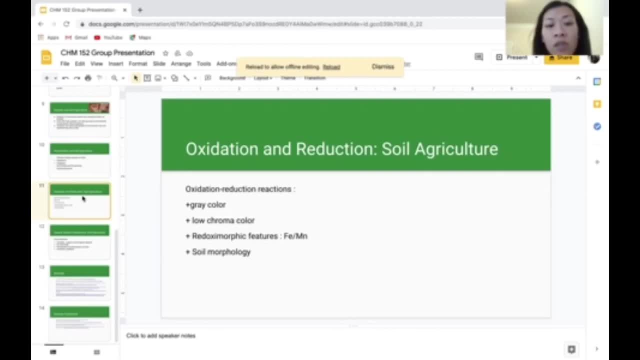 the soil have different color, So the red color. they have very poor nutrition, low chroma color. Let's talk about the organic matter interaction in soil agriculture. So the availability of trace elements to plant is governed by a variety of reactions that include complexation with organic and inorganic ligands.